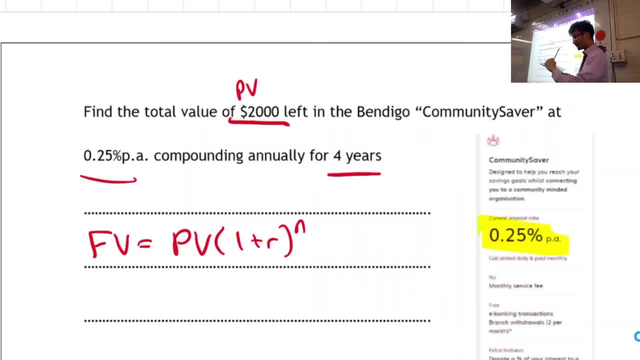 So I've got my present value, what it's worth right now. I've got the rate and I've got n the number of periods right, But the r, though, right if you look at the r. what did I say, Ben, about the r? 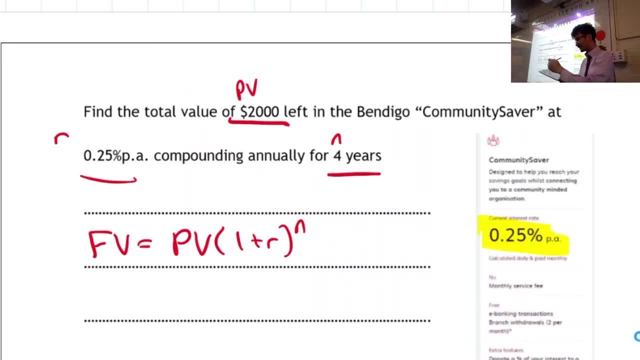 How do I want it? actually, I don't want it as a percentage right now. Yeah, I want it as a decimal. yeah, So what's 0.25%? 0.25% as a decimal. well, you can convert that. 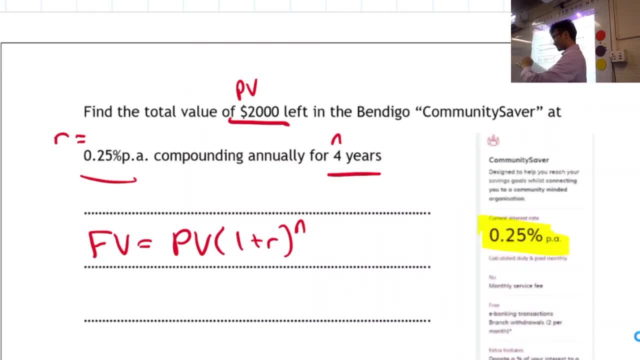 And what would that be? Yeah, you just divide it by 100.. Okay, See, there's nothing that's changed here. These are the same thing. but there's a particular reason why I want it written like that, and I'll show you in a moment, right. 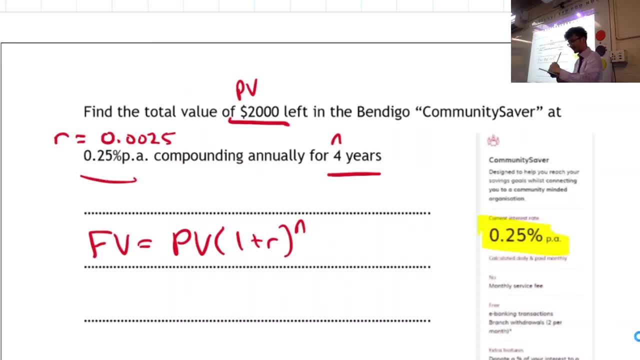 Because now when I'm putting this into my formula, my calculation to calculate the future value, I actually want to put that in my calculator, right? So let's go ahead and do that. I've got my present value 2000.. 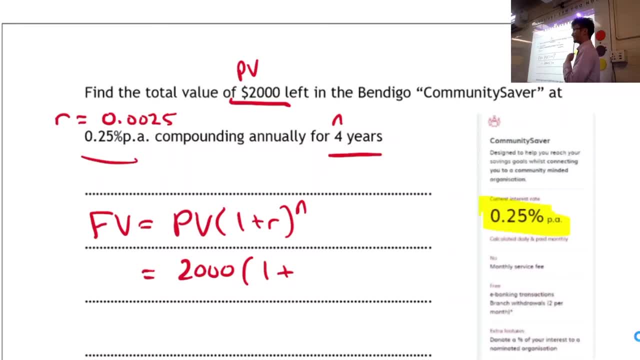 Times 1 plus, and this is why I want this rate as a decimal, Because if I put it as a percentage it's a bit harder to put in your calculator. I want you putting it in your calculator like this: Okay, Bailey and I need my number of years, and then Bailey's going to calculate that for me in a moment. 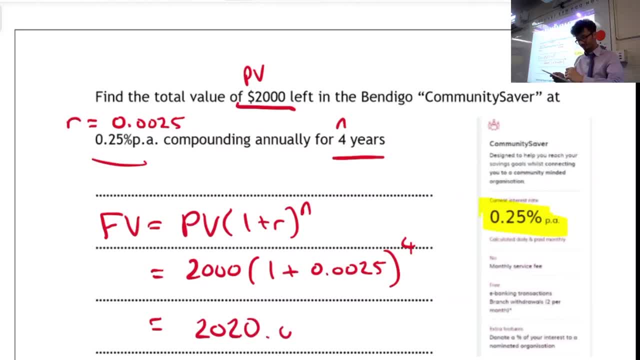 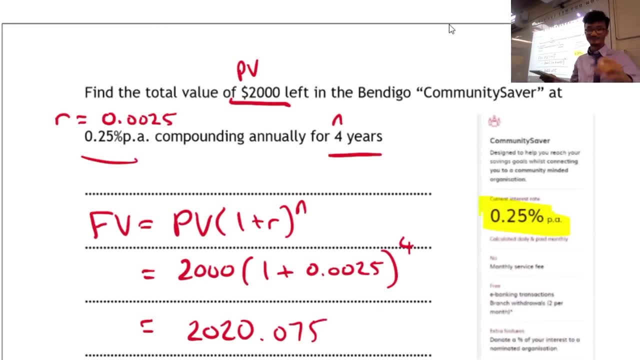 2020. 2020. 0.5, cool, So I guess the interest rate leaves a little bit to be desired. Now, typically with these answers, we'll round them to what we say, the nearest cent, right? 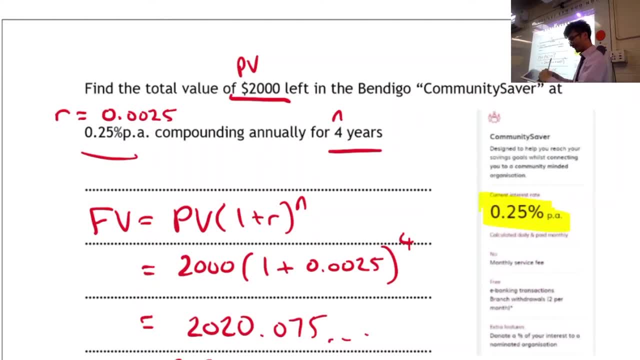 So that's two decimal places, So 2020.08 dollars. there nearest cent Future value is this: How do we get more money? How do we get more extra amounts? There's a few ways you can do it. 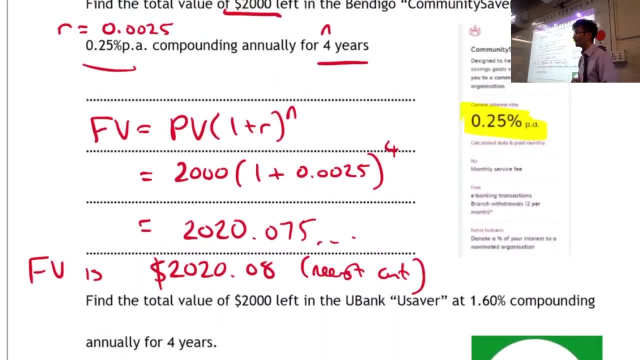 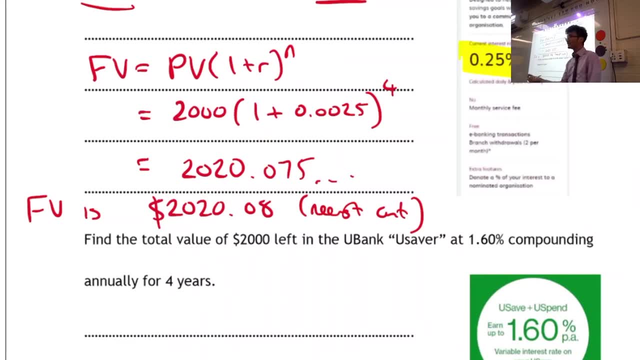 Sorry, What was that? He said how to get more money. Yeah, How do we get more money through legitimate means? There's a few ways you can do this. You can change the principle or we can increase the rate. Now, this is a bank called UBank. 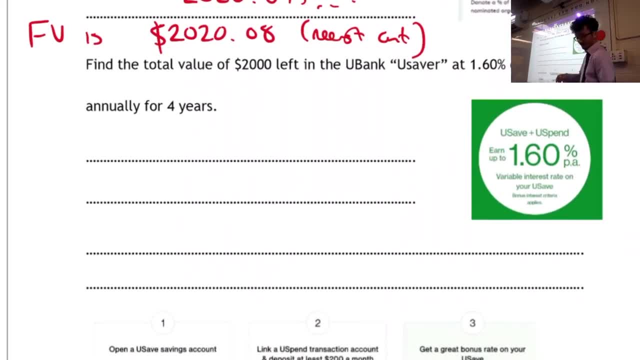 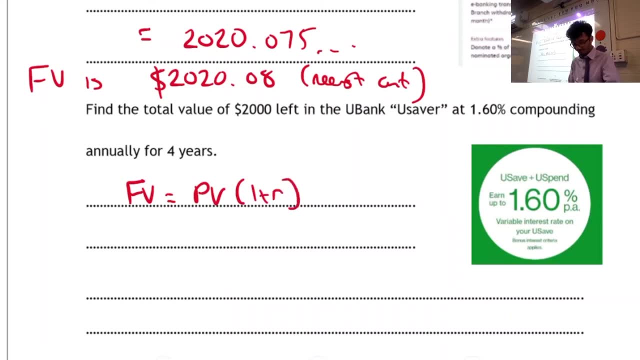 And so they have a better rate here- 1.6%. Let's see how much better it is. Let's use the same formula: Same thing, same information. Let's see how much more we get just by increasing. Let's see how much more we get just by increasing the rate a little bit. 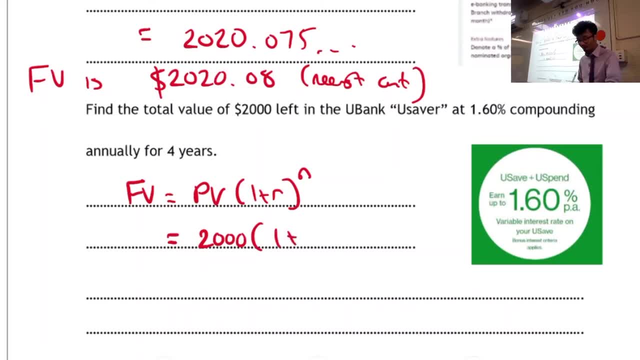 Before I do that, I'm still going to write down all the information that I have. But again, I want this rate here as a decimal. Bowen, can you help me out? What would this rate be as a decimal? So I'm looking at the rate here. 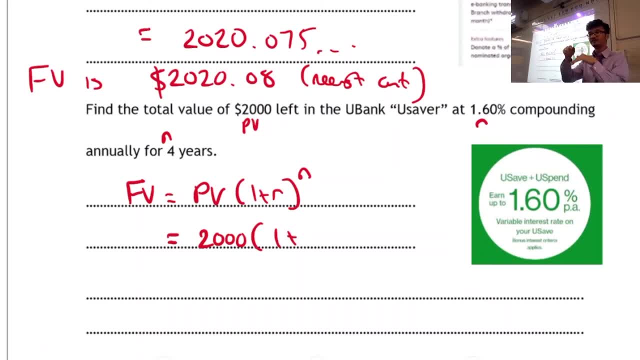 I want that as a decimal actually, because when I put it in my calculator, I want to type it in as a decimal rather than as a percentage. It would be 0.016.. Yeah, 0.016.. Good, So then that makes it easier to put in your calculator. 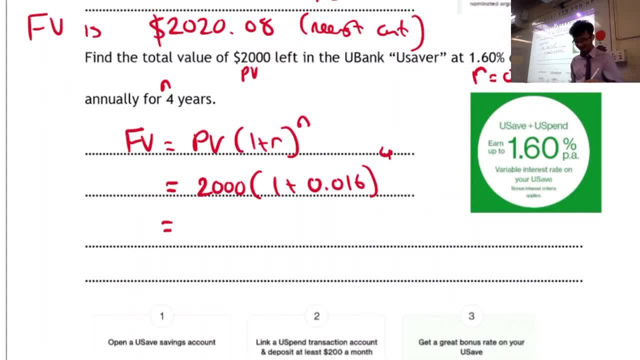 Do we get a little more $11.. Oh, that's not bad. What was your final answer? Yep. So we say the future value is $1,131.10.. What I did one before, No, Thank you. 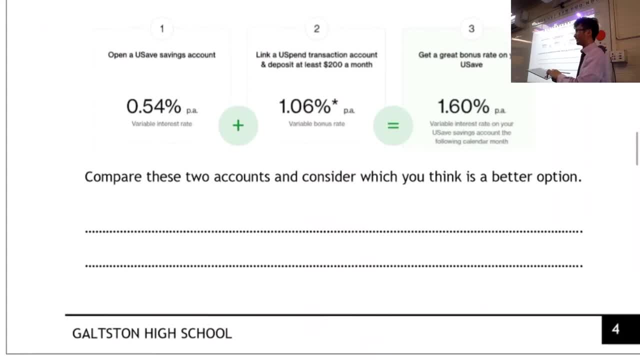 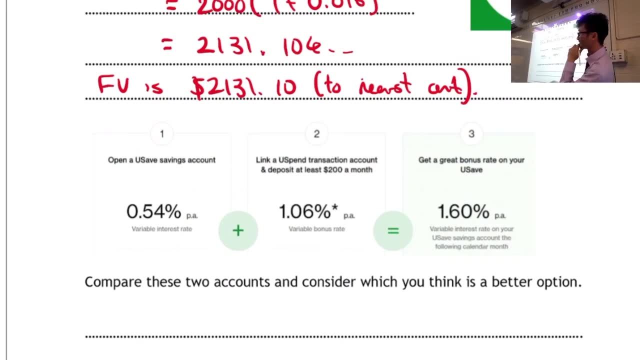 Just as a follow-up question, guys, This is not really like a math question, I suppose, but you can have a think about it. Rhys, what do you reckon? Which account would you say is better? The second one? The second one, because you get more money, I guess, right. 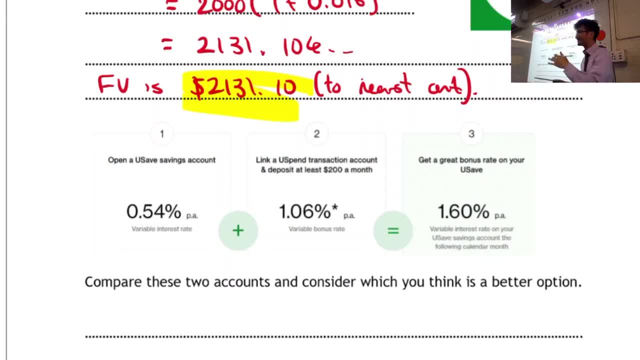 And there's an argument to say: yeah, the more money you get, the better. But typically- And this is just more of like a life lesson for you guys- Typically when you get more money, there are conditions applied to it, right? 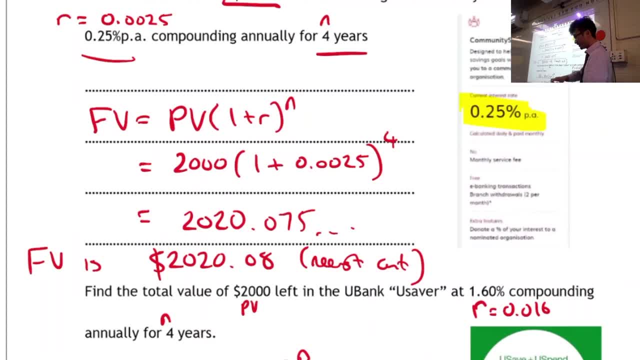 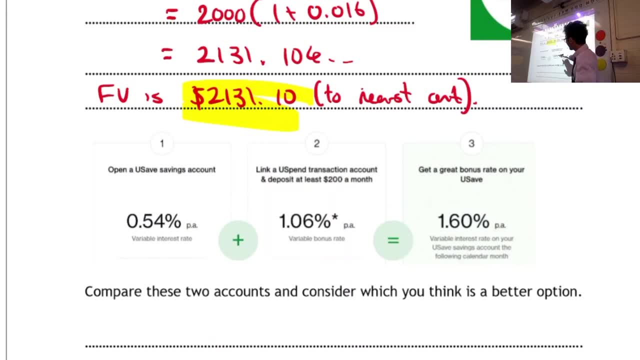 For example, the Bendigo one. that's kind of for a good cause You're giving back to the community. With the UBank one, there's actually some conditions for how you get this extra interest, Because actually what you have to be doing is you also have to be depositing $200 a month. 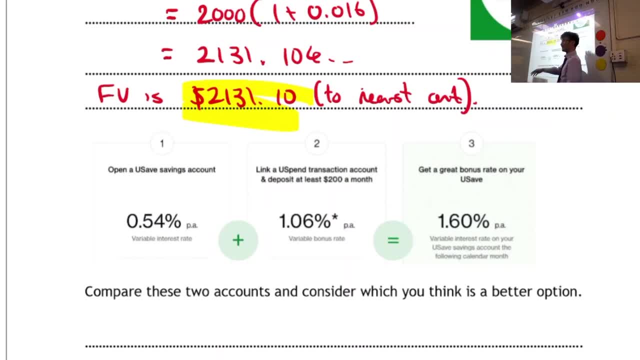 to get this bonus interest right. Without it, you're not getting the full rate, And so just watch out for these kinds of calculations that sometimes they require you to deposit certain amounts Or spend certain amounts. so Are you trying to sell this to get us to?